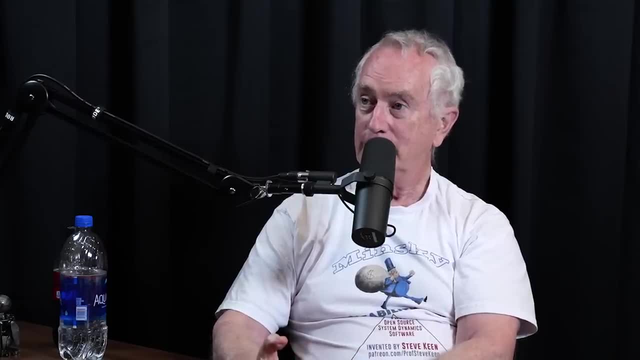 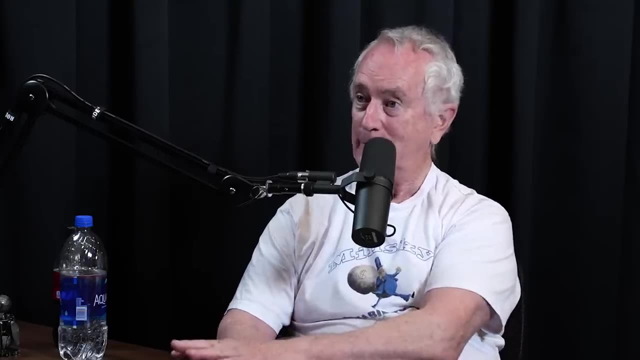 Is bad. Yeah, I'd say: learn system dynamics. Do a course in system dynamics which you can apply in any field, and then apply what you learn out of system dynamics to the issues of economics, if that's what interests you Get a base engineering education. 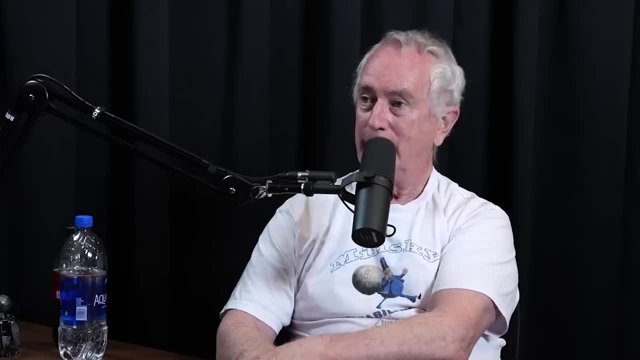 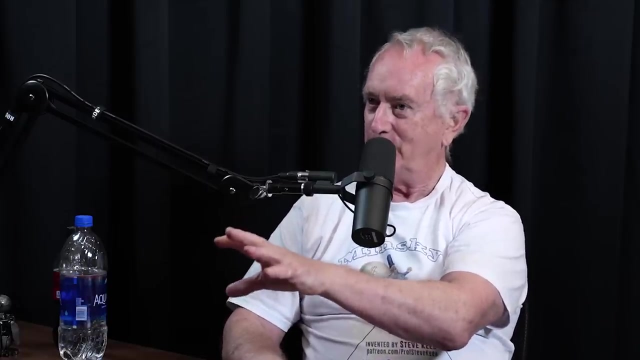 Yeah, a base engineering education. That is far better than doing an economics degree. In terms of life, my life is pretty chaotic in many, many ways. My friends and family will tell me that every opportunity. I'll tell you an example of a really funny incident. 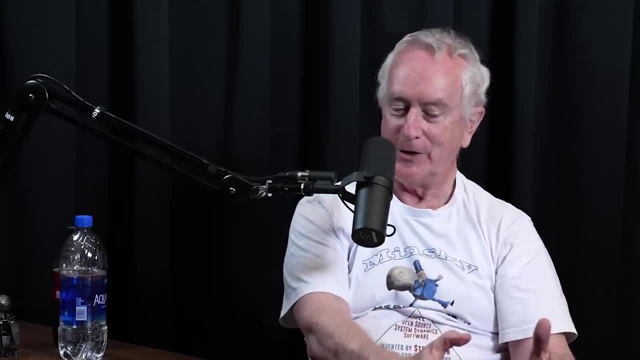 that occurred to me because I led the student revolt at Sydney University, as I mentioned, when I was 20 years old- Yeah, this is great. And then, in my, I think, about 28 or so, I went to a restaurant one night and I found 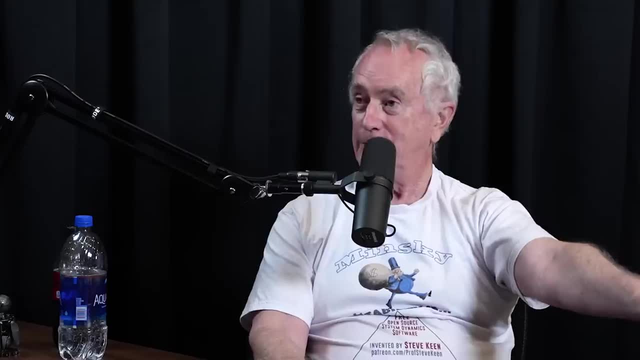 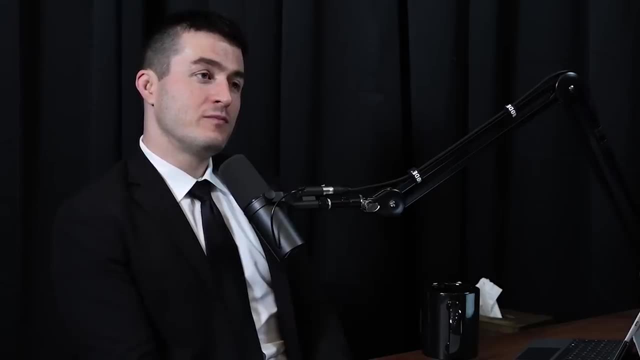 a bunch of guys- all guys who'd done accounting at the university but had also been part of the student revolt, So they hadn't seen me for about a decade. and they said: what have you been doing, Steve? And I talked about what I'd done. so I'd been a school teacher. 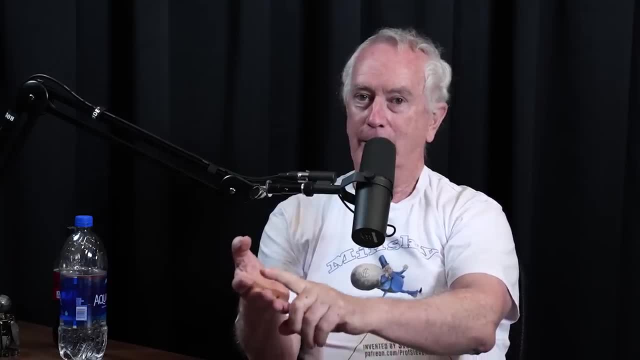 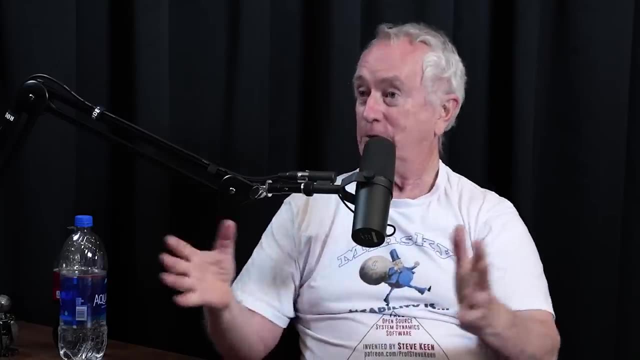 for a while. I then worked in overseas aid. I was doing computer programming at the time and I'd forgotten what else I was doing at that point, so I explained it to all of them And they were at a Bucks night, one of them having a wedding coming up the next week And one 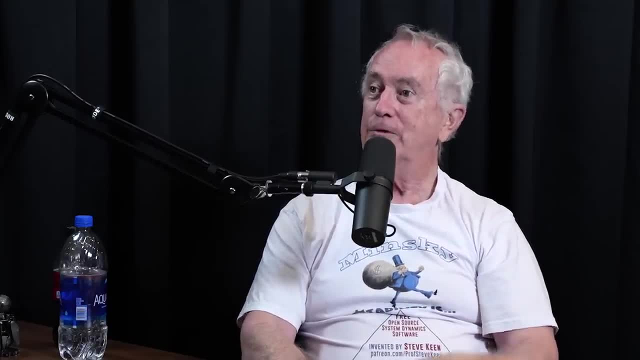 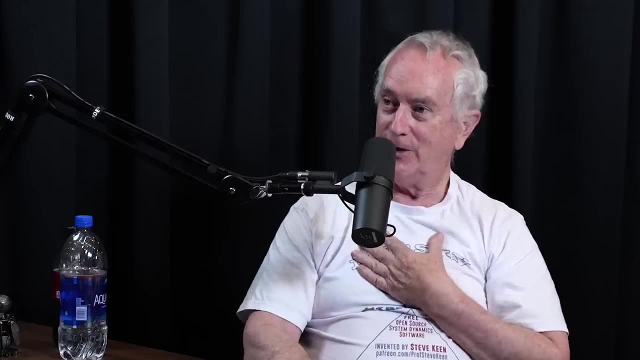 of them said I wish I'd done that, And there was silence around the table. It was obviously silent agreement And I looked at them and said: hang on, guys, Look at the downside of my life. You're getting married. I don't even have a girlfriend right now. You've got. 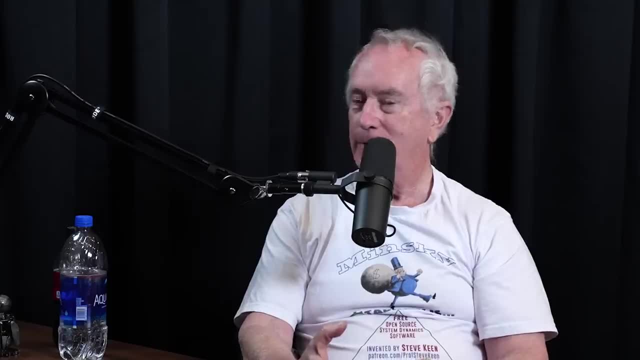 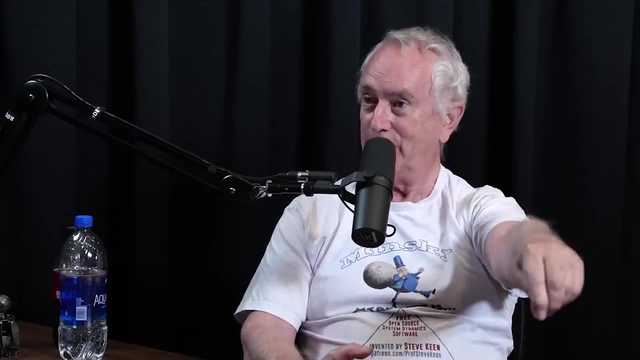 all got secure jobs. I'm unemployed. You own a house. I haven't even got a car. Look at the downside of my life. And the bloke who was the kingpin of that group- a very innovative bunch of guys in the student revolt. So he said, Steve, we would still all rather. 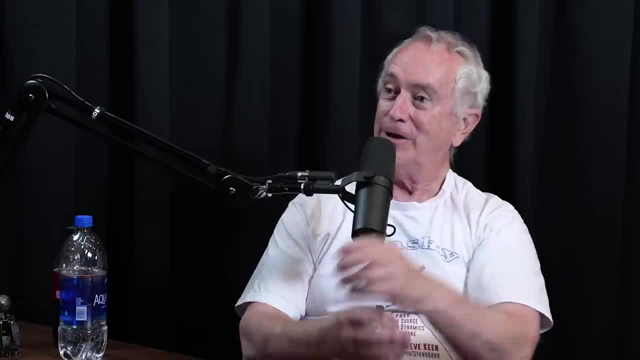 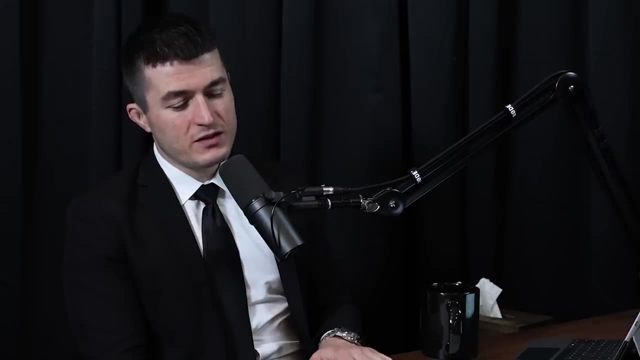 have done what you have done. And they did accounting because it was safe, Always get a job. They were bored, shitless. Wait, did you have a sense that the chaos you're always Jumping into was dangerous, Or was it just the pull of it that?